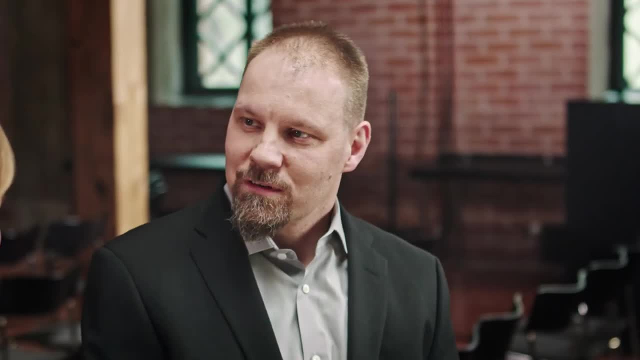 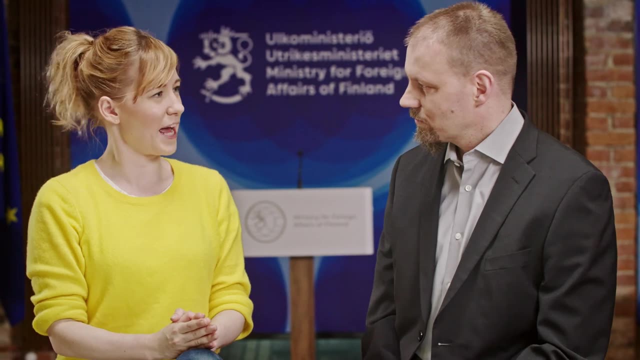 And who told you about this attack? Who was the secret messenger? It was another foreign state, A friendly one. After the notification, what were the next steps? What happened within the organization here? Well, first, I skipped the lunch, Makes sense. 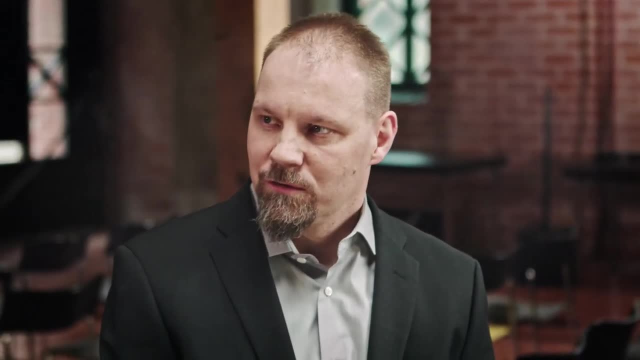 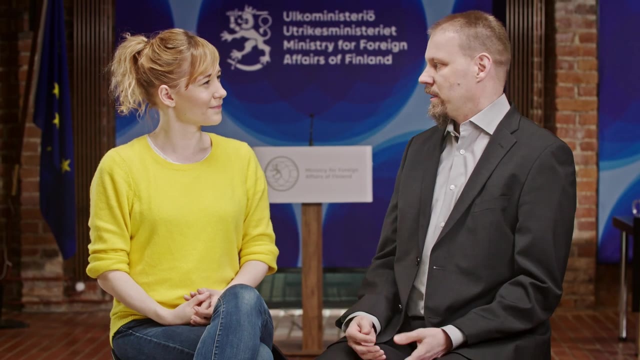 And then we went to a security operations center And we took out our network flow And then we were looking for those facts or data which were written in that document that I was keeping, And how long, at this point, the attack had been going on. 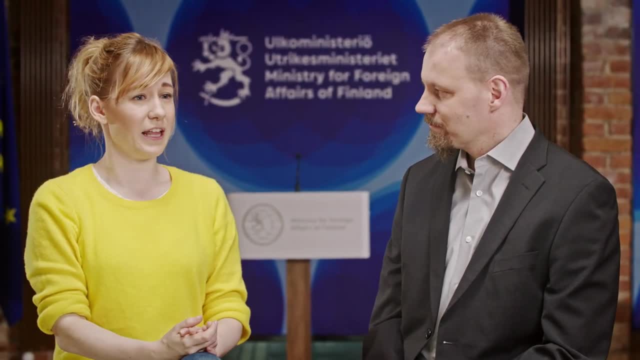 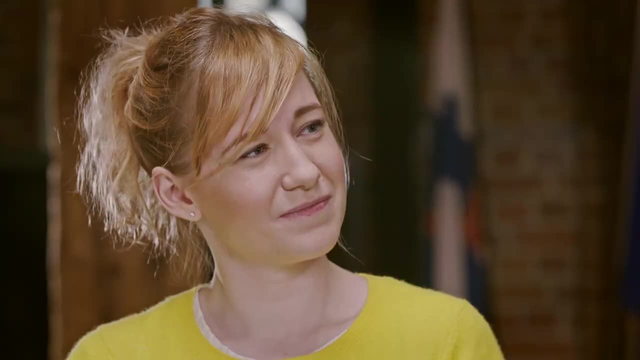 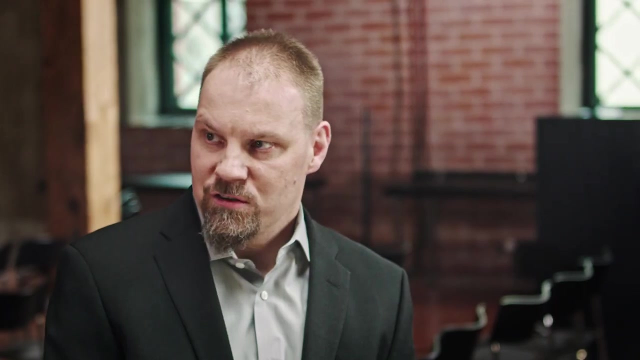 At least four years. Four years, Wow. And what kind of response did you have to the attack? How long did it take to solve the issue? Well, the first response took one hour. We blocked that flow And in a couple of months we had an understanding how the attacker was operating in our network. 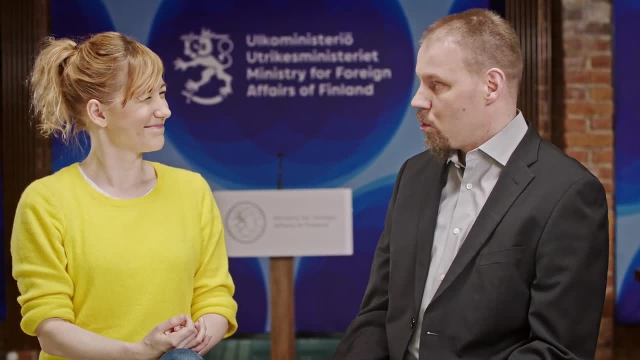 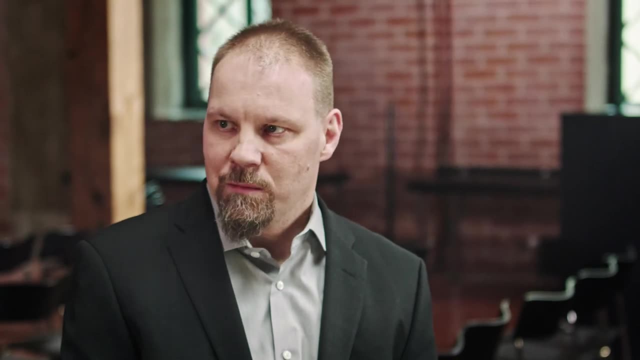 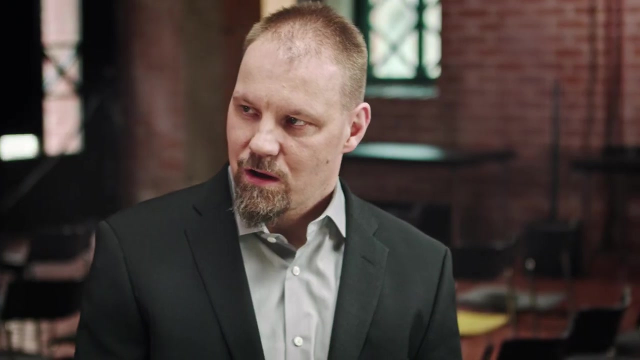 And then we started to raise our shields more than before And we enhanced our surveillance in our network And after six months, we made our own counter message in one day. So, during these days and weeks and months, how did you feel Well to understand that we've been breached? that was my worst day of my work life. 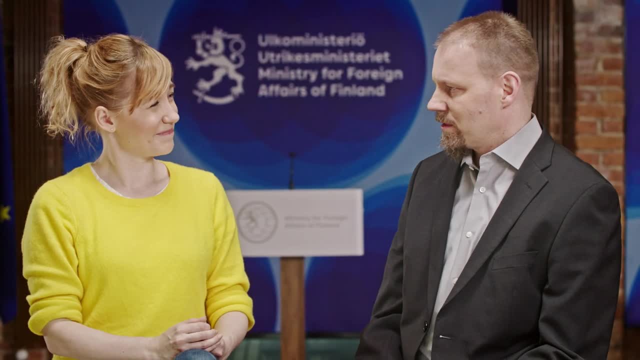 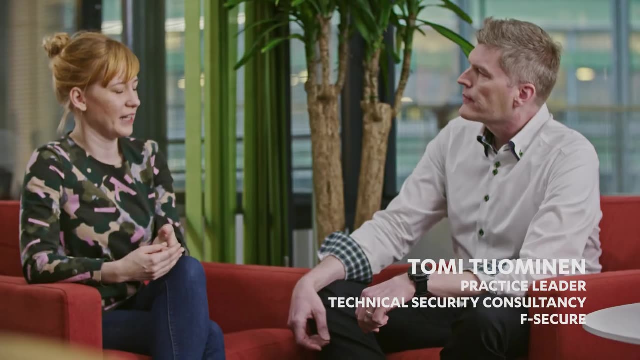 Why is that? Well, to find out that something that you've been taking care of, that you have well, didn't succeed. What happens when, within an organization, when an attack is done? Well, usually nothing, because they don't know that they've been targeted. 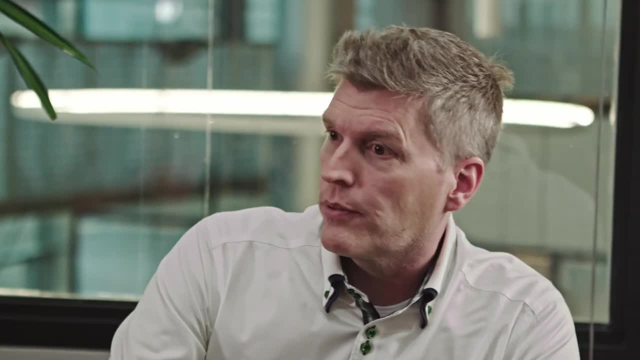 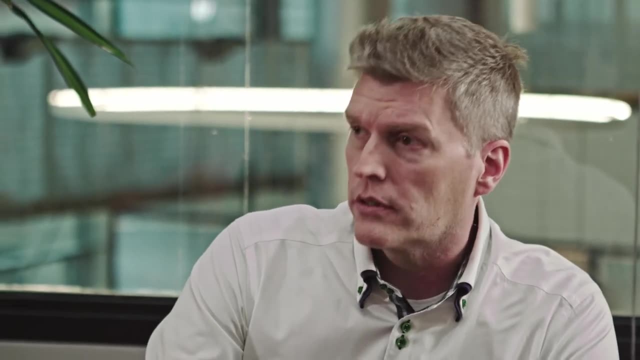 But once they discover it, the most common response is panic, Because it's usually a situation. it's like being mugged: You're not really prepared. If you're an average person, you're not really being prepared for being mugged. 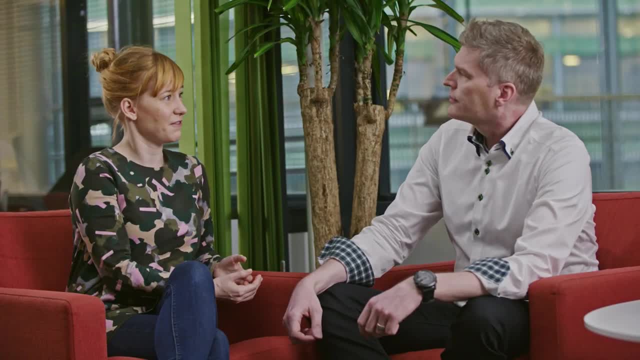 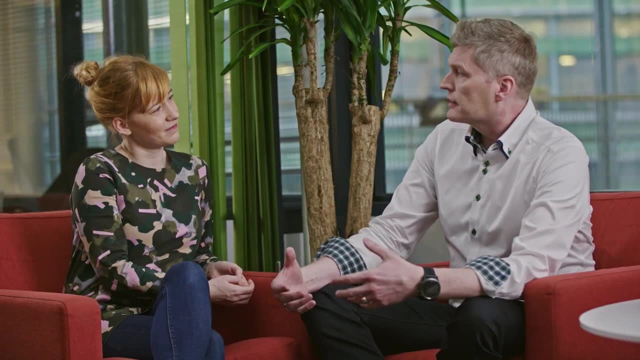 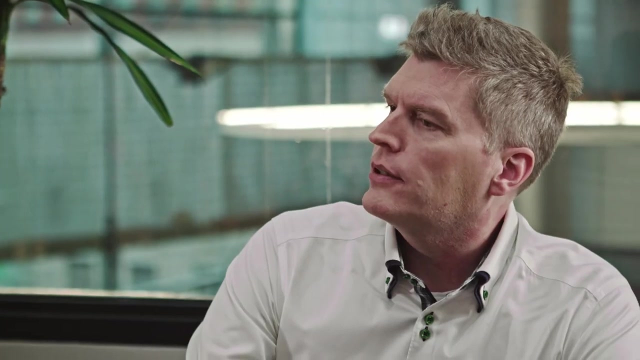 And is there something an organization can do to defend themselves against an attack like this? Absolutely The only advantage defender has is that they were there first. If you know your environment, if you know your target infrastructure, well then you know what you have and then you can defend against it. 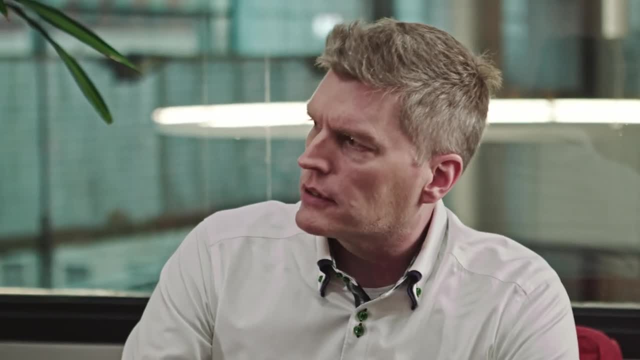 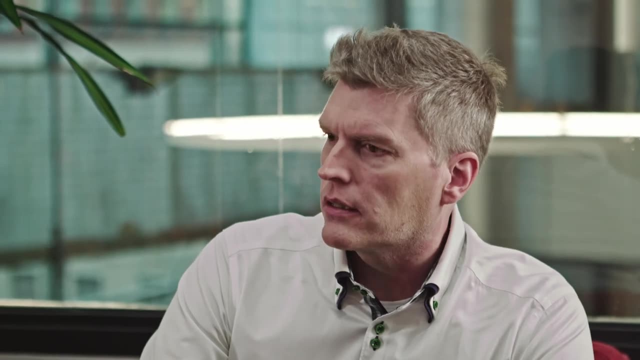 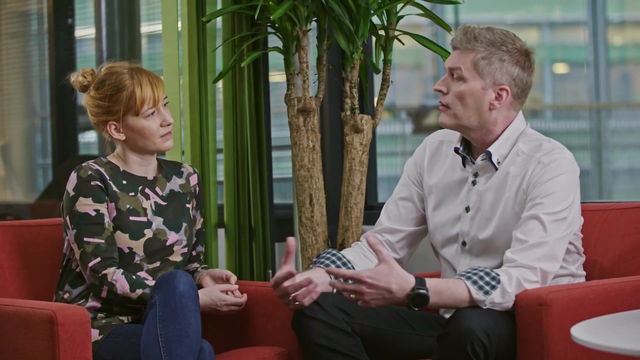 Once you go past the exploitation phase- so we go to lateral movement, we go to data exfiltration phases- the chances for an attacker getting caught increase every second. So that's where the defender advantage is, So you don't have to play fair. 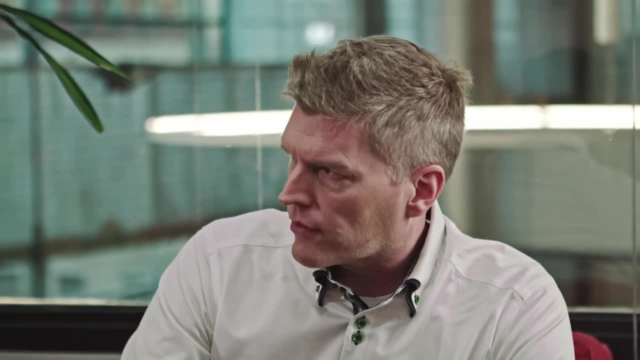 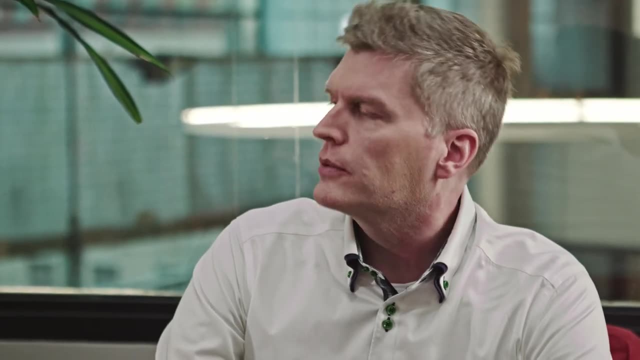 So you can booby trap your organization, You can booby trap your infrastructure, You can put honeypots in there, You can add visibility, and so on. So there are a multitude of things that you can do. You've worked in a lot of different industries. 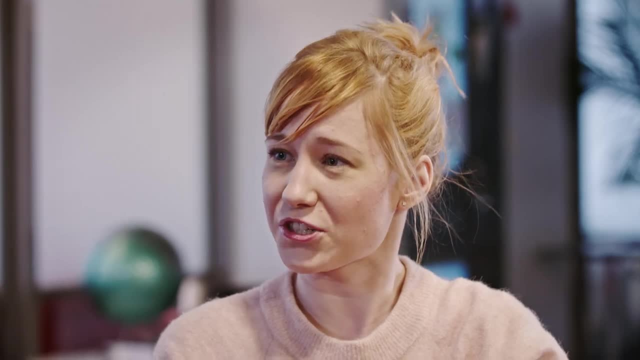 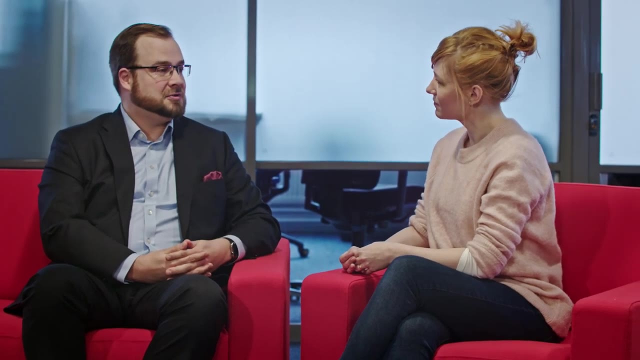 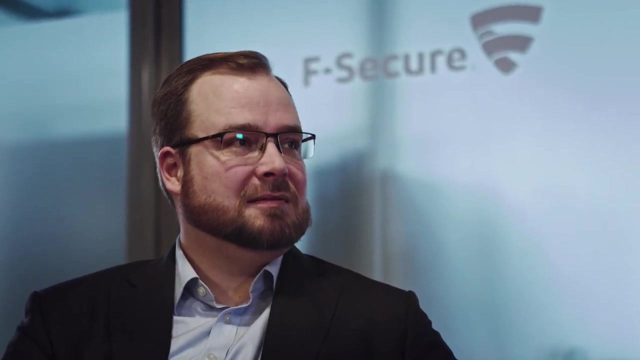 In your experience? how prepared are companies for breaches like these? On average, not very well prepared, Especially if you're not a company in well-regulated industries or not a critical infrastructure provider. They tend to have these preparedness procedures in place and run systematic rehearsals. 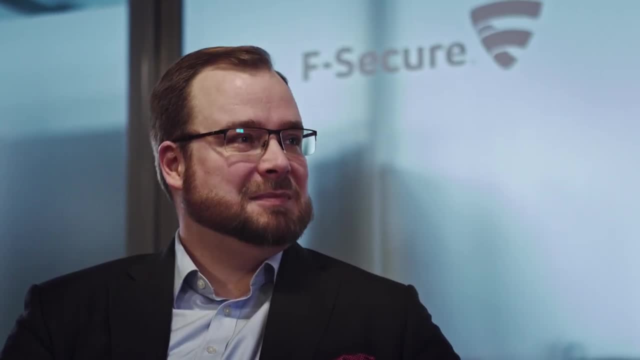 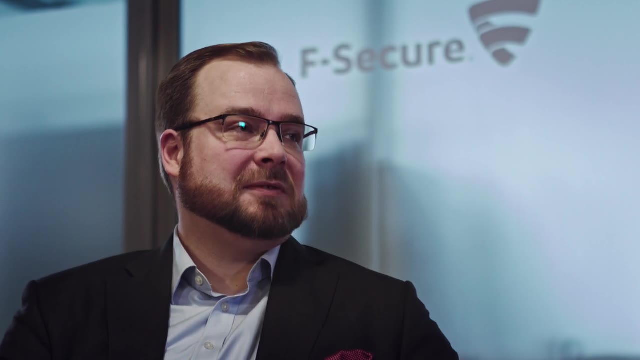 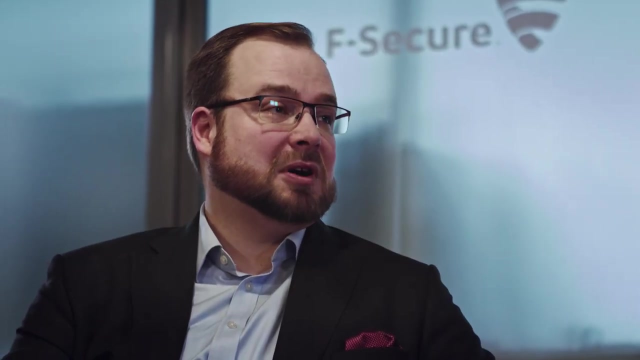 An average company, you may have a crisis management team, typically your top management, but you don't run rehearsals, especially on the field of cybersecurity. And what are the risks a company who is not prepared might face? There can be a multitude of consequences for a company when they eventually face a breach. 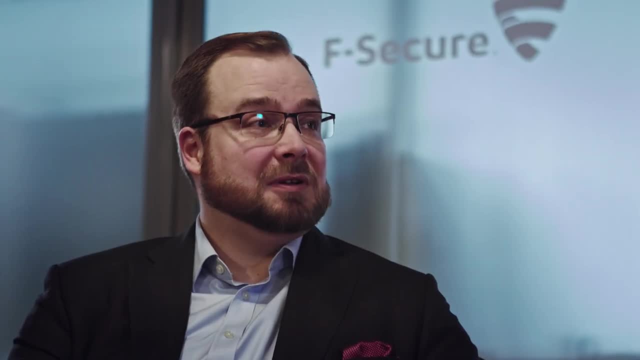 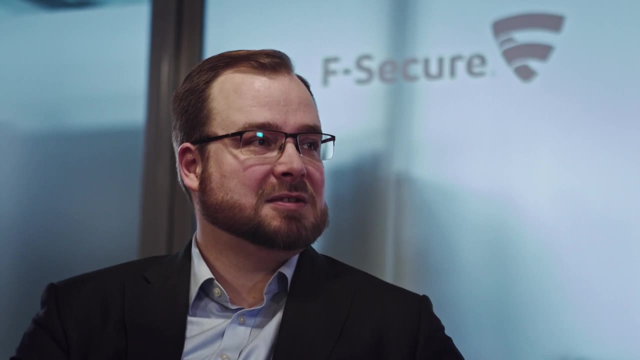 One that is most often discussed is the reputational impact. So you're bound to lose the respect and trust from your stakeholders, your owners and customers, and that's going to hurt you in the long run. But there's a multitude of other consequences as well. 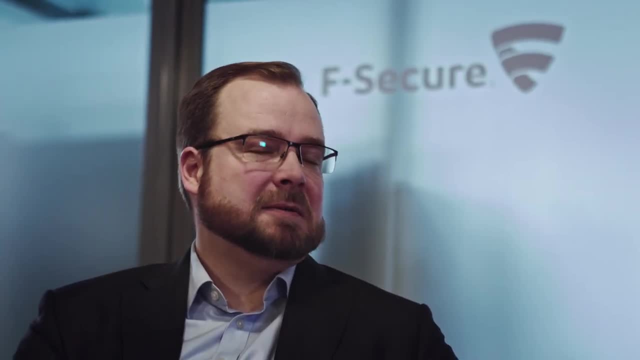 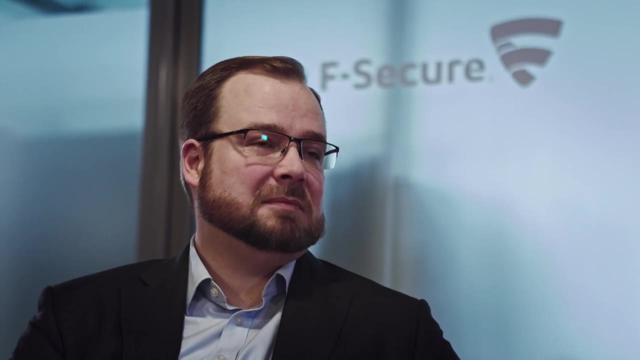 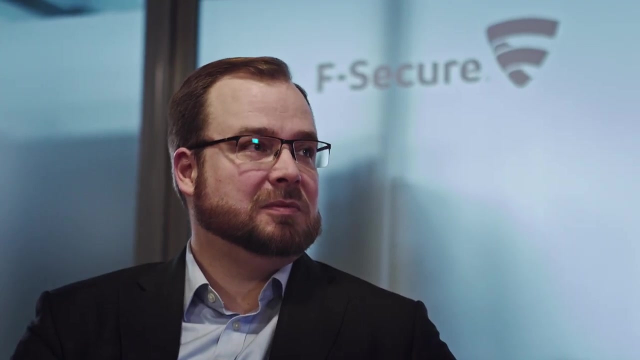 You might need to pay damages fines. There could be productivity impacts, revenue losses. So it's really a difficult situation for many companies, And what you should really pay attention to is that your response is very accurate and effective, So you can at least try and limit some of these consequences. 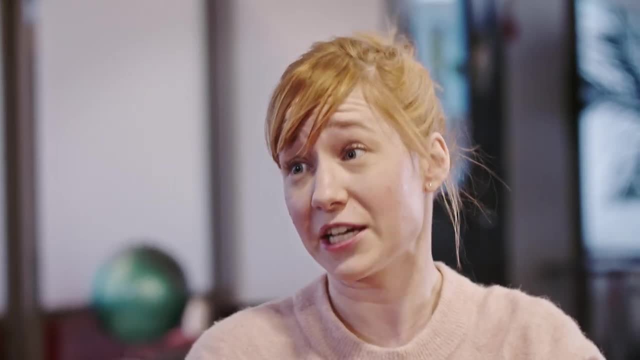 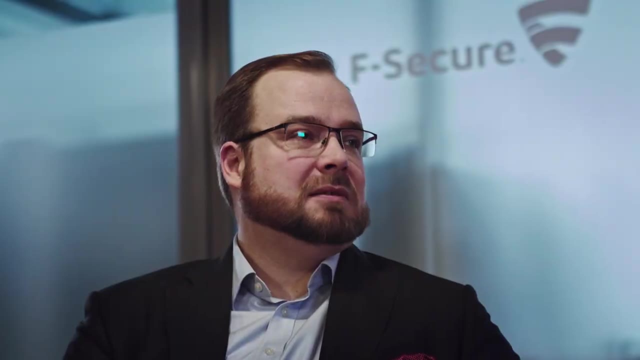 How do you create, within an organization, a culture where security is everyone's business? Well, one of the first elements is, of course, awareness, So your employees should be aware of what is the critical information, what is the information and data that's sensitive, confidential to our business. 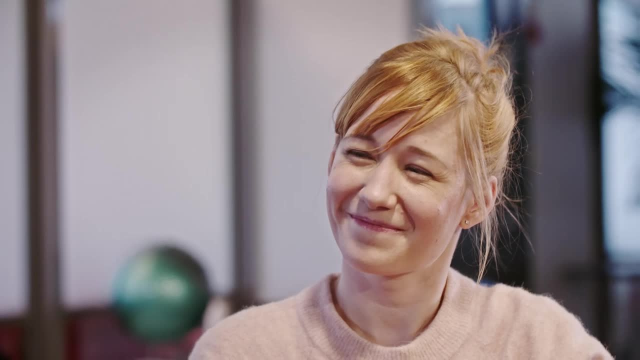 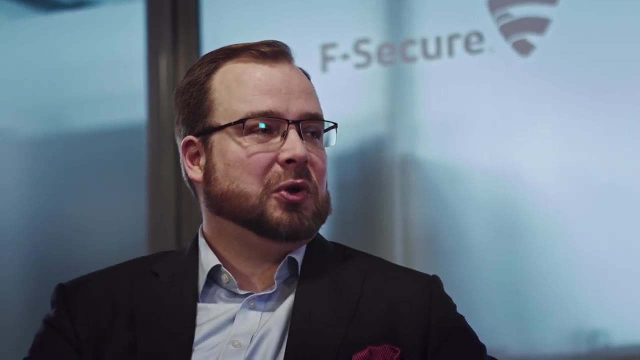 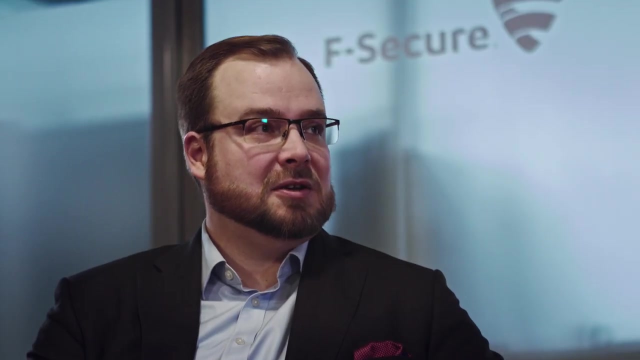 Then you should create a culture of mutual trust. You should teach all your employees to recognize potential security problems and report them. And if you treat your employees as the weakest link of security, it's difficult to build that trust. I mean, they might not tell you if they clicked a link or opened an attachment.